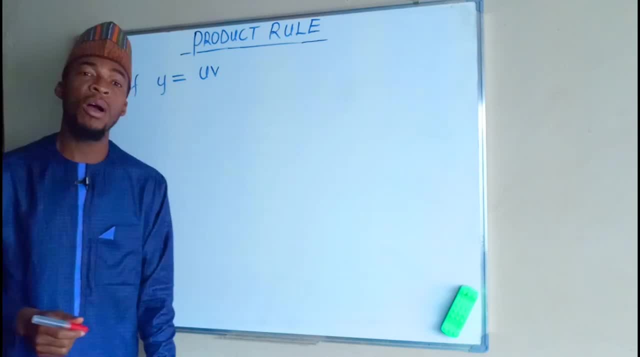 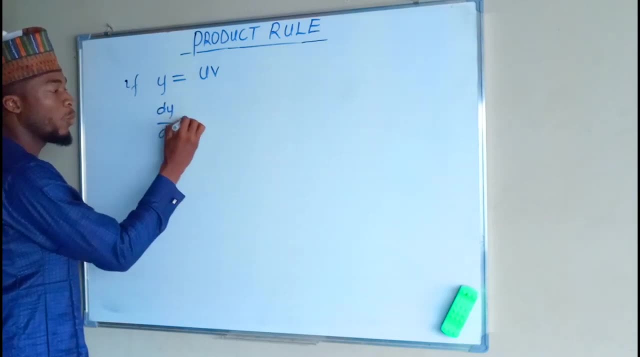 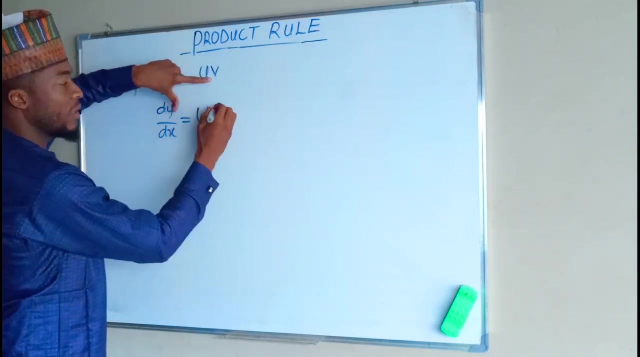 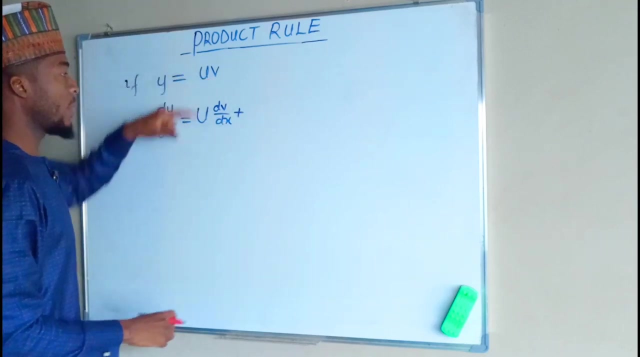 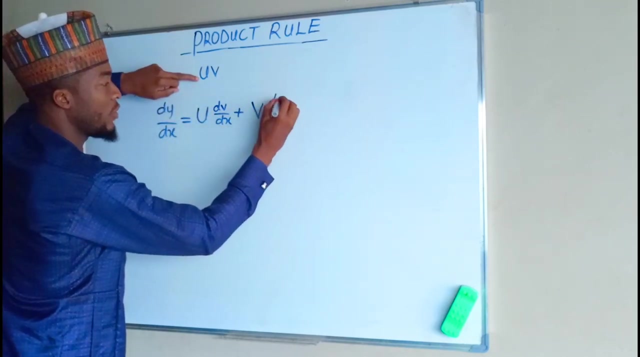 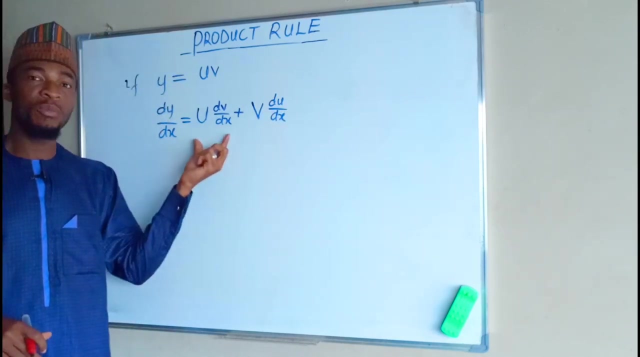 times v, where uv, a function of x, dy, dx will be equal to. If u constant, differentiate v dv over dx, plus If v constant, then now differentiate u du over dx. You can write this one right before this, because addition is commutative And this formula for product true- is being derived from the first. 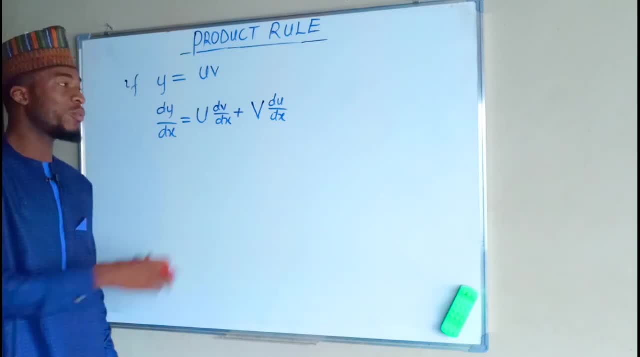 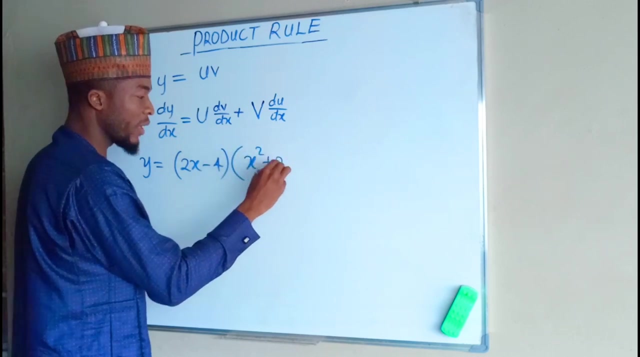 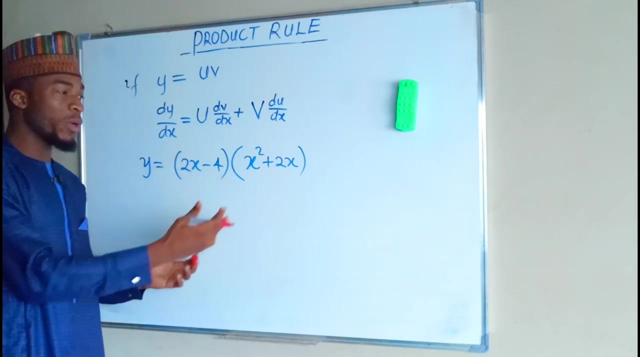 principle too. If time permits, I'll show you how to prove this. So force y because 2x minus 4 times x squared plus 2x. There are two ways in which you can differentiate this function. First, you can expand the bracket, and secondly, you can apply this: 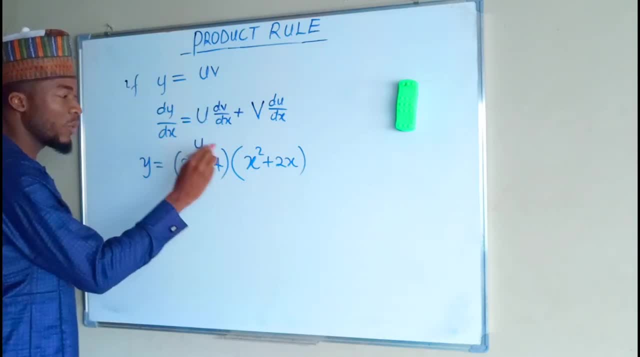 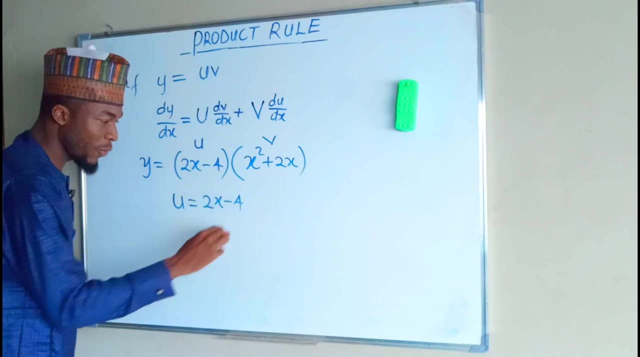 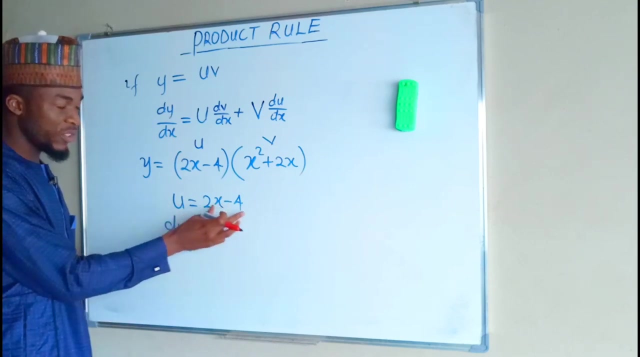 rule which says that you can let this to be u while this to be v. If u equals 2x minus 4, then du over dx will be equal to. We differentiate this algebraic term. Start out with the first one, which is the first term is 2 if you differentiate it minus. 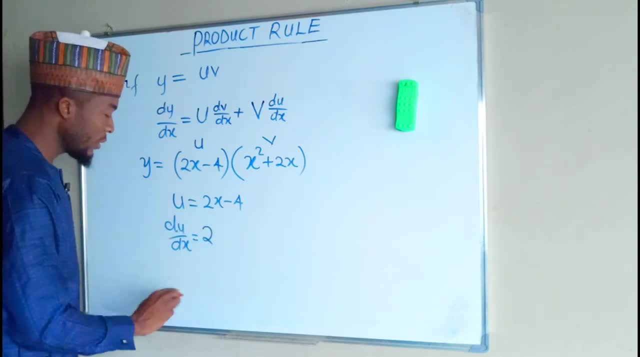 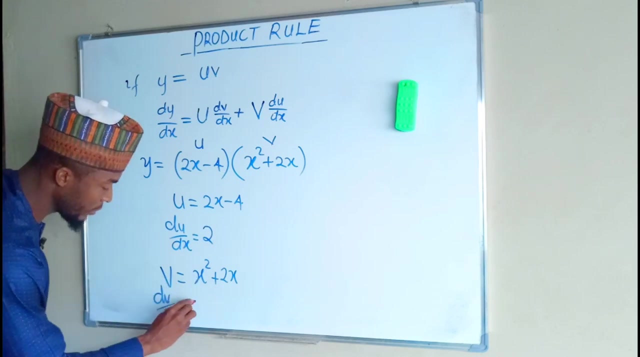 0, because the derivative of a constant term is zero. then v equals x squared 2x. dv over dx will be equal to: If you differentiate this term, you will have 2x plus. if you differentiate other time you are going to have only two. now let us substitute into this: 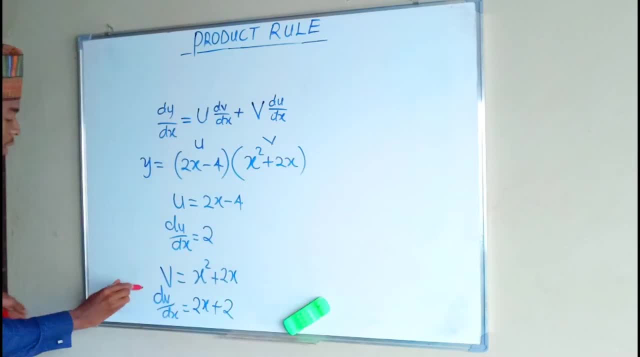 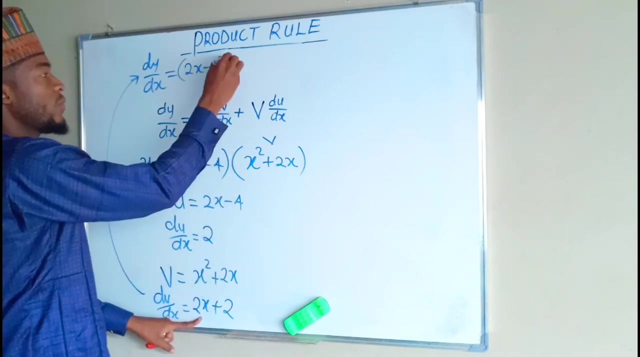 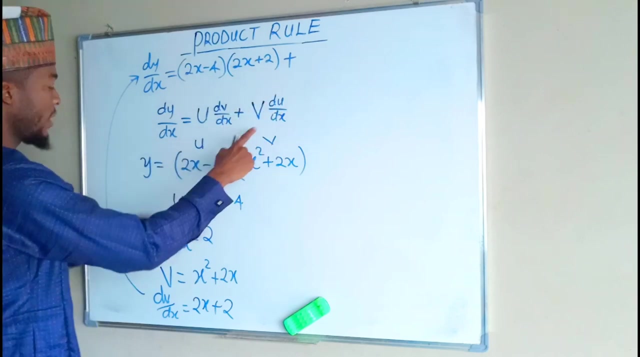 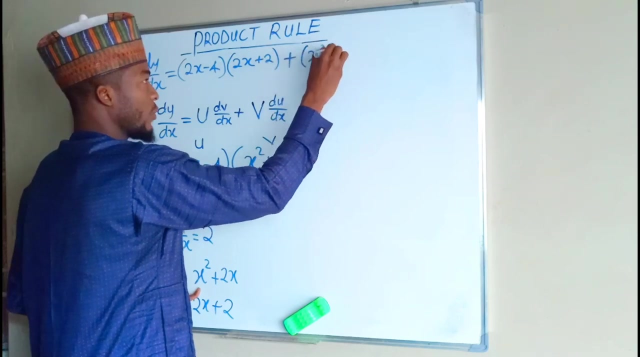 formula dy over DX will be equal to you, and now you is 2x minus 4. 2x minus 4, DV over DX is 2x plus 2, 2x plus 2, then plus V, our V is x squared plus 2x, x squared plus 2x. 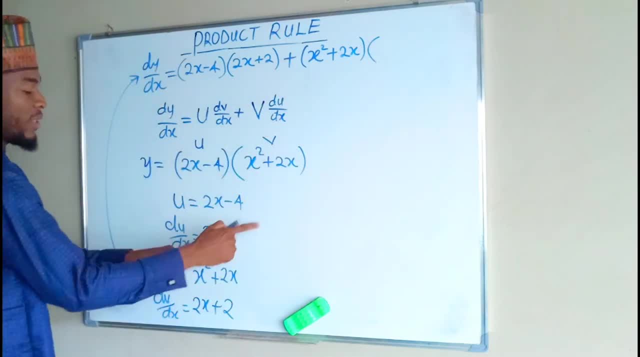 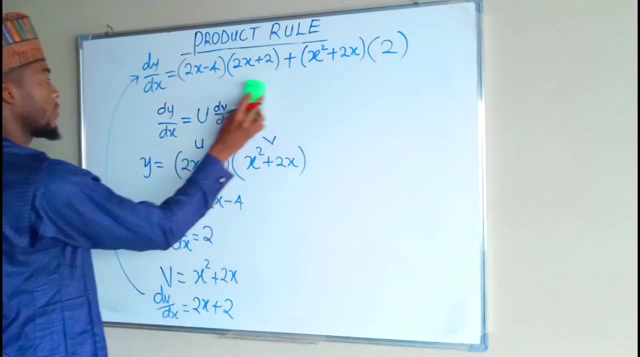 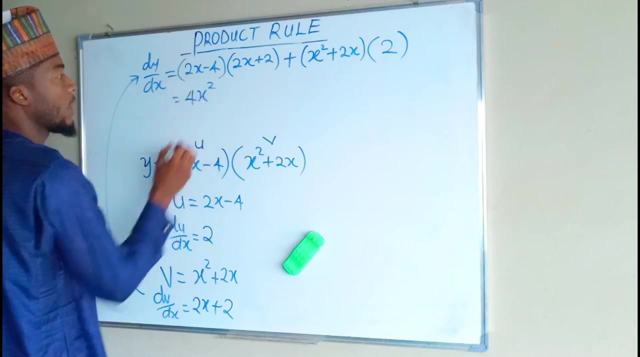 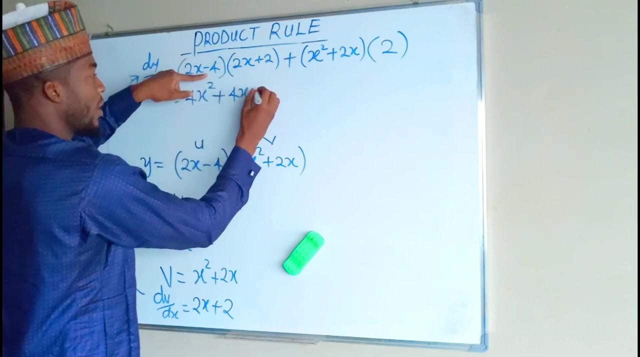 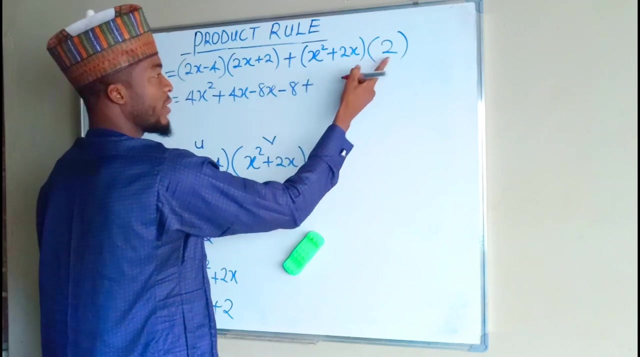 times the u over DX, which is 2. now let us expand each of these brackets. this time, this is 4x squared. this time, this is 4x minus 4 times 2x is minus 8x minus 4 times 2 is minus 8. then, plus x squared times 2 is 2x squared plus 2x. 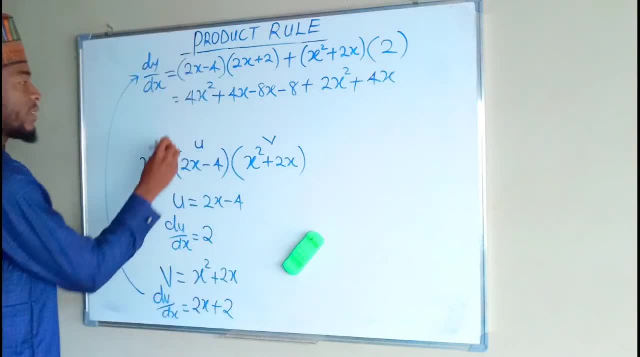 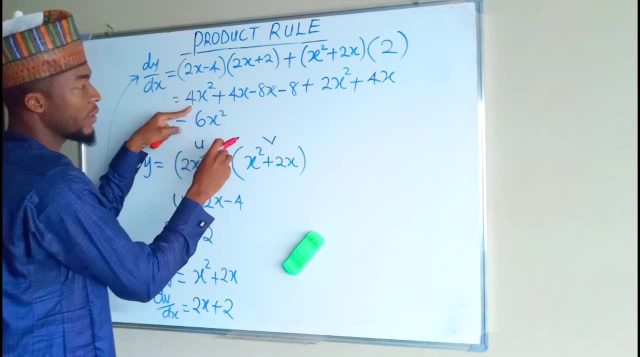 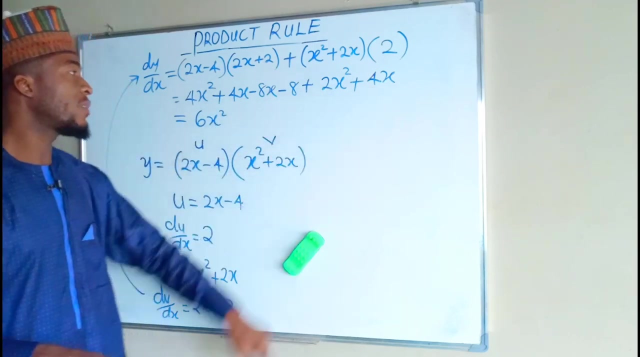 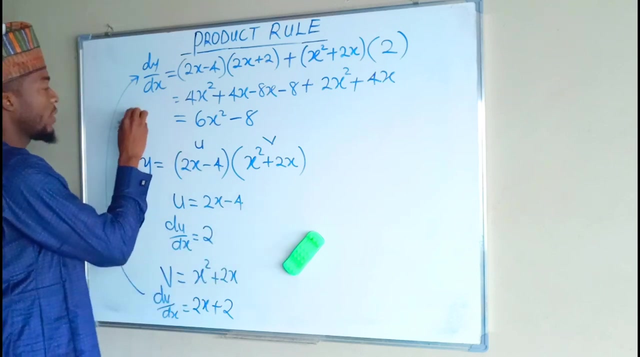 times 2 is 4x. now let us collect the like terms together: squared plus 2x squared is 6x. squared 4x minus 8x is minus 4x, then minus 4x. plus 4x is 0, then minus it. therefore, dy over DX is equal to 6x squared minus 8. 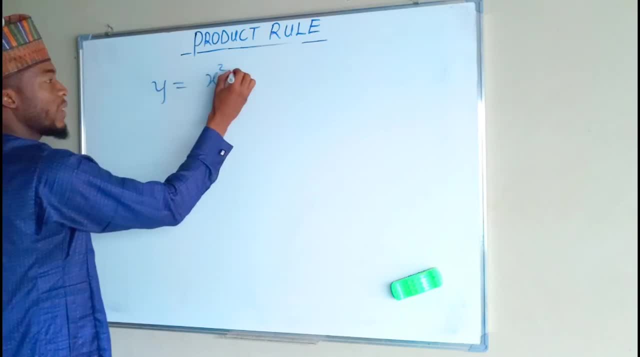 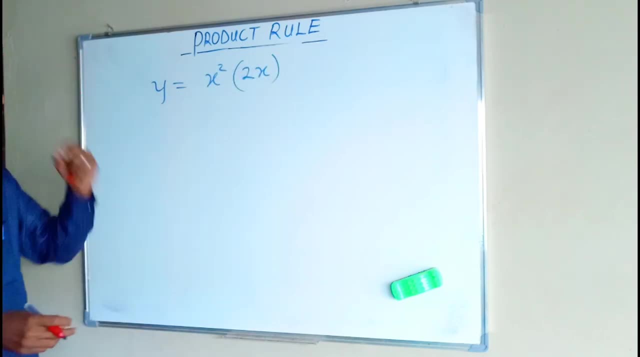 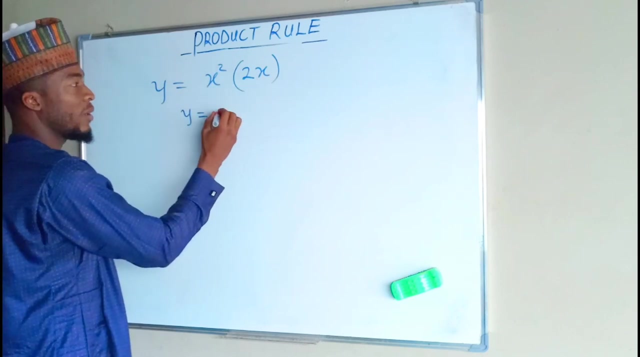 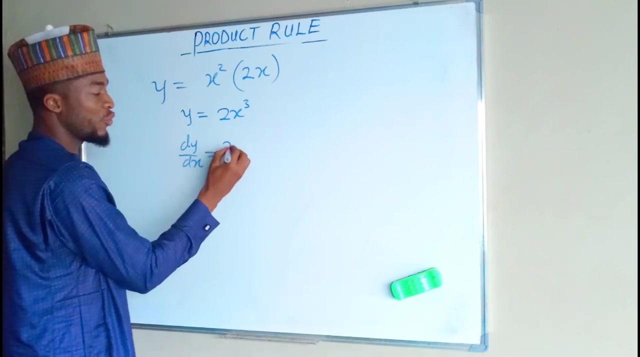 suppose y equals 2x squared times 2x, and this is what you have first of all. if you like, you can expand this bracket. you know Y will be equal to this time. this to X cube. the DUI over DX will be equal to 2, the we differentiate the function X, the times. 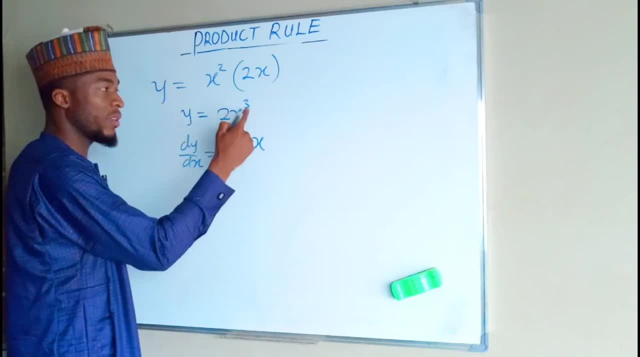 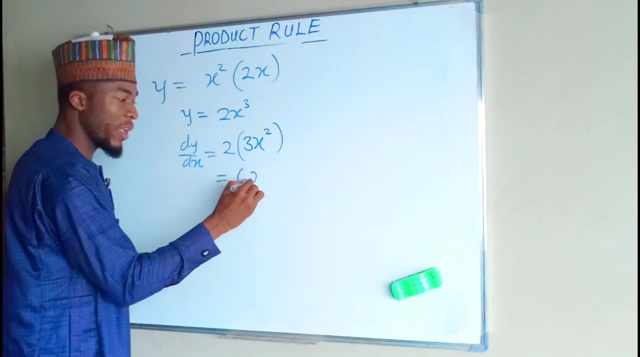 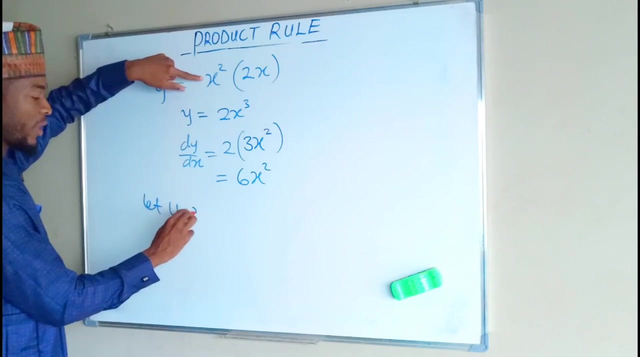 the x by the exponent, which is 3x, and you subtract one from the exponent 2, then this will be equal to 6x power 2. now let's apply product rule and see: let let u equals to x power 2. du over dx will be equal to 2x. let v be equal to 2x dv. 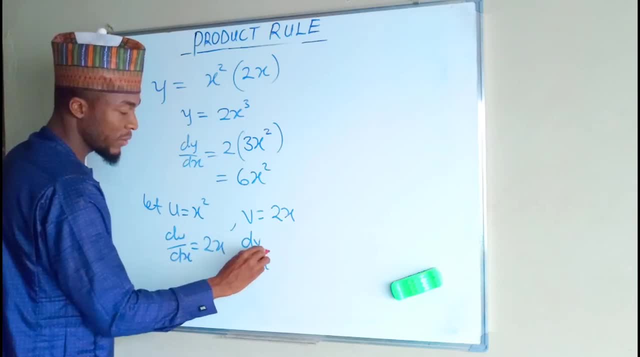 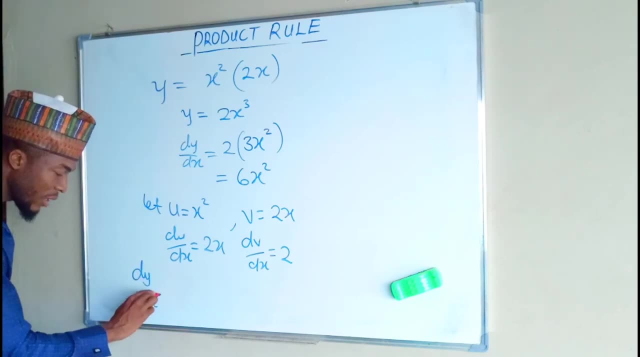 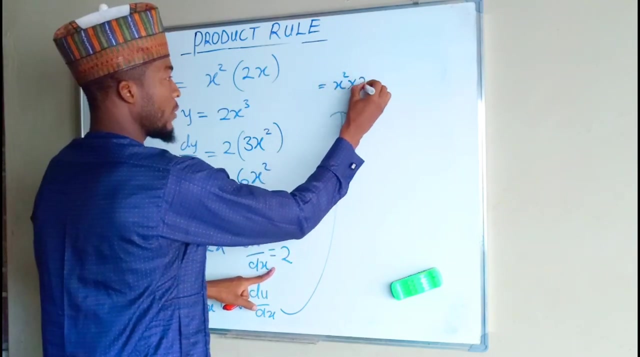 over dx will be equal to 2.. now, using the rule which says the y over dx is equal to u, then dv over dx plus v, du all over dx. this will give us, you know, that u is x squared. dv over dx is 2. then plus v, you know v is 2x. 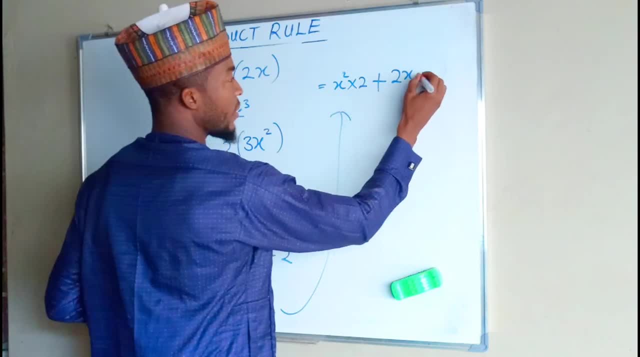 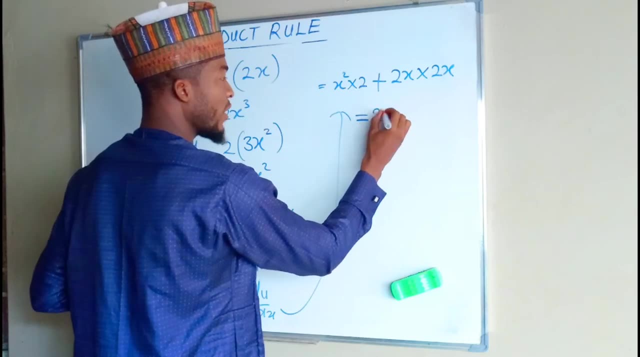 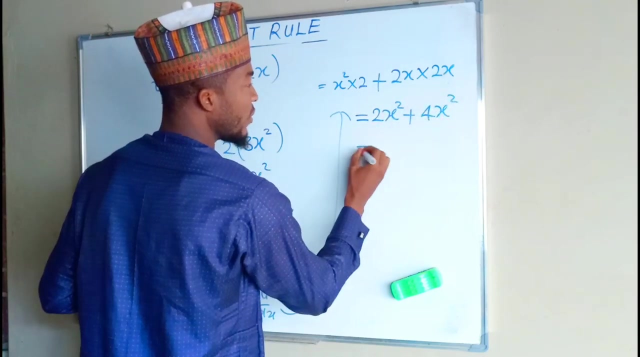 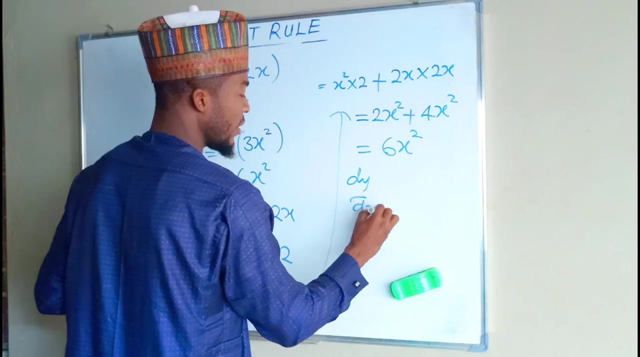 du over dx is 2x x squared. times 2 will give us 2x squared. plus 2x times 2x is 4x squared, this altogether equal to 6 x squared. therefore, dy over dx is equal to 6x squared, which is just equivalent to this. 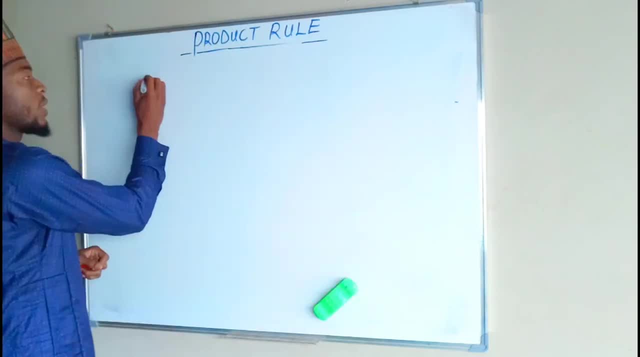 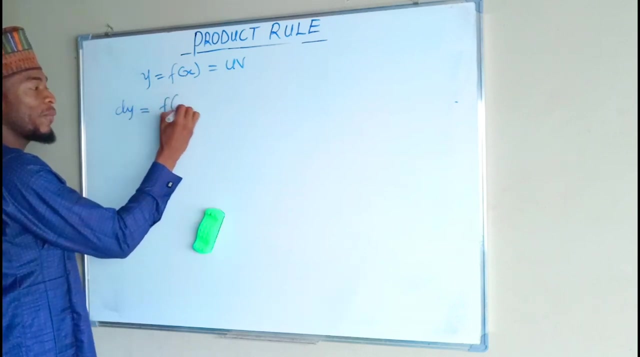 so where do we drive this formula from? if y, which is a function of x, is equal to u times v, u and v are functions of x, dy will be equals to f of x. if y is equal to f of x plus dx, minus f of x, 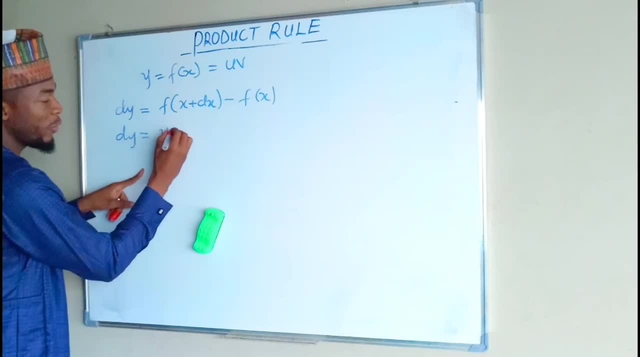 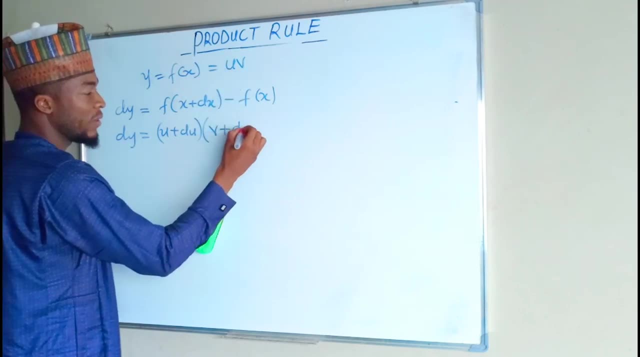 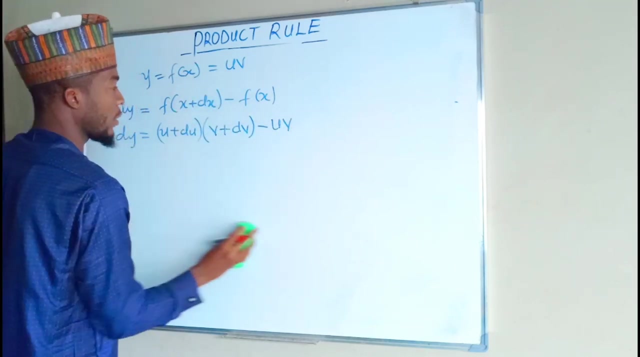 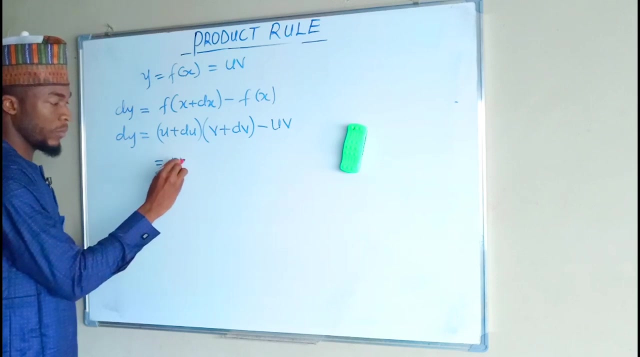 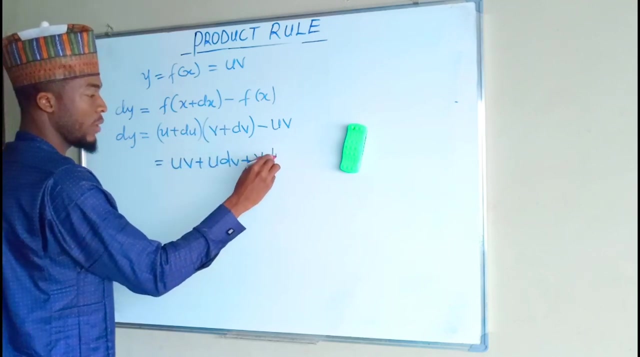 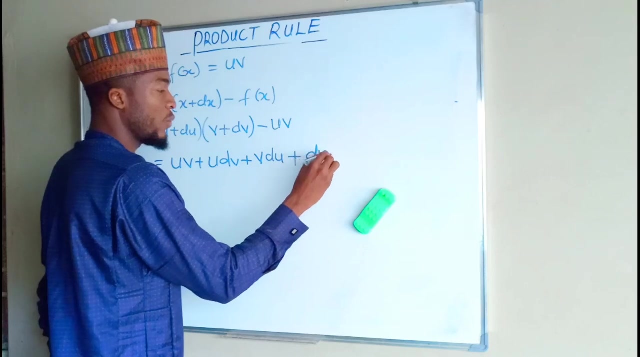 dy will be equals to. since u is a function of x, you say what u plus du and the other term v plus dv minus f of x and f of x is uv. So if you expand this times u times v is uv, u times dv is udv. Then the other term du times v is vdu plus du, times dv, du dv. 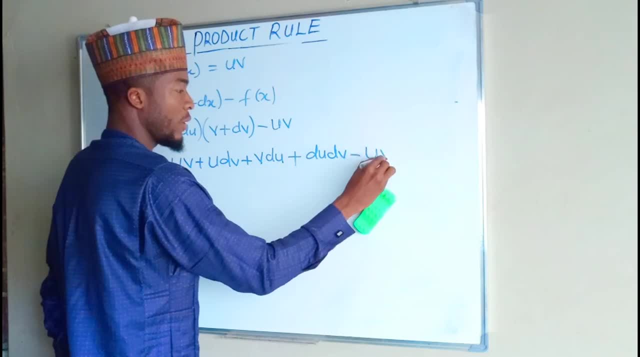 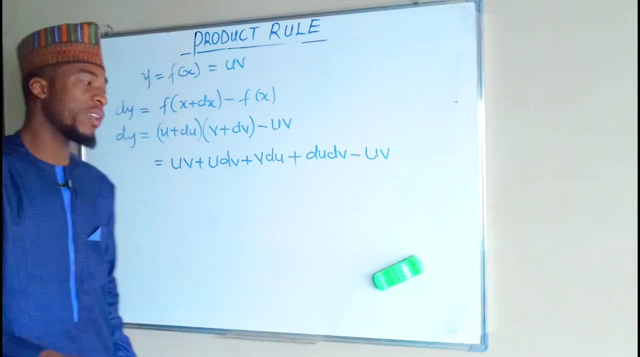 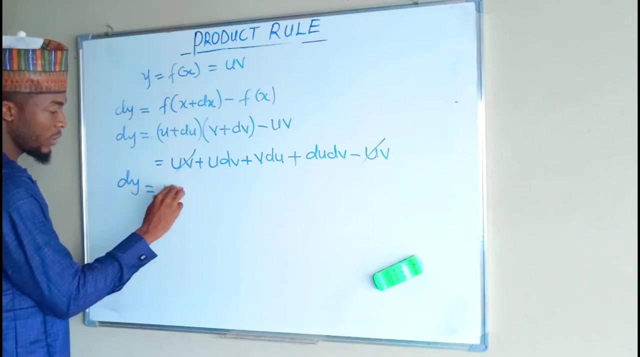 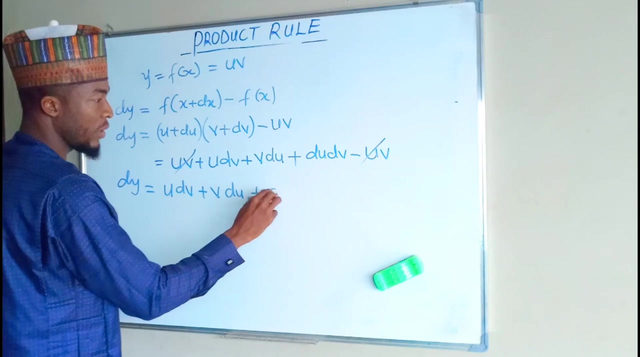 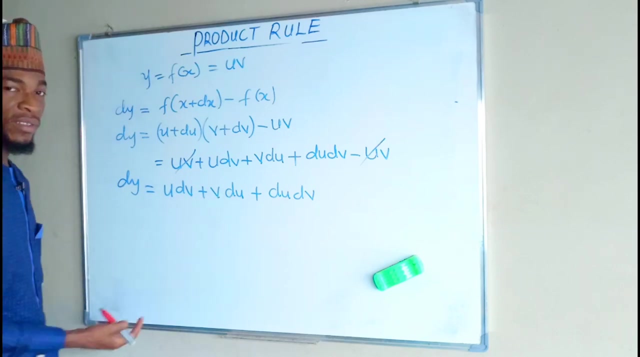 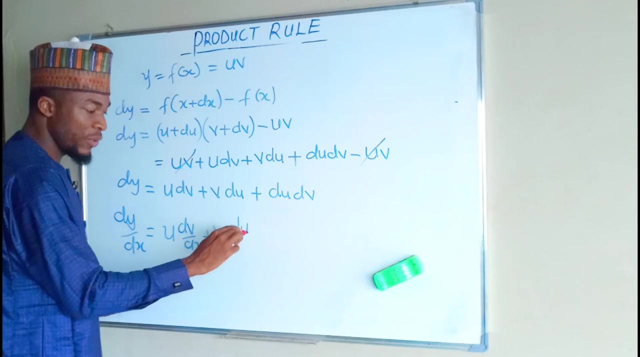 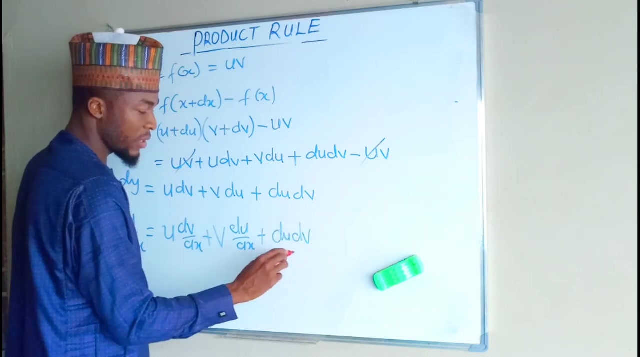 Then minus uv, uv. We have uv here which is positive and we have another uv which is negative, so they cancel out. dy will be equal to udv plus vdu plus du dv. Now we are going to divide each of these terms by dx. Therefore, dy over dx will be equal to udv over dx, plus vdu over dx plus du dv all over dx. 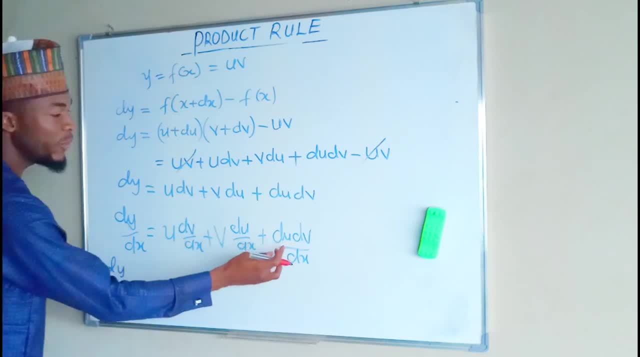 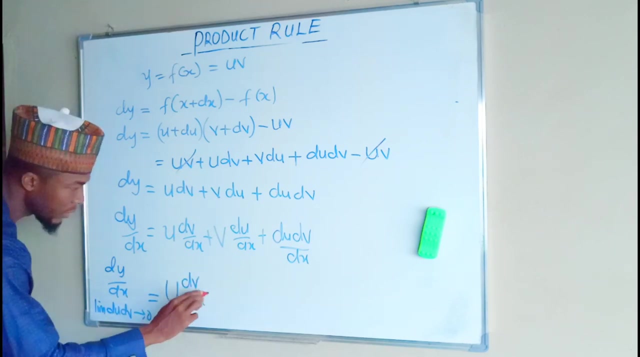 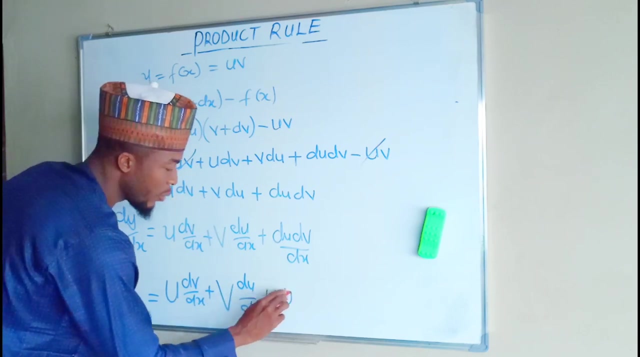 dy all over dx. As the limit of du dv approaches zero, limit du dv approaches zero, will be equal to udv over dx plus vdu over dx plus zero, Because if du times dv is equal to zero, divided by dx will be zero. 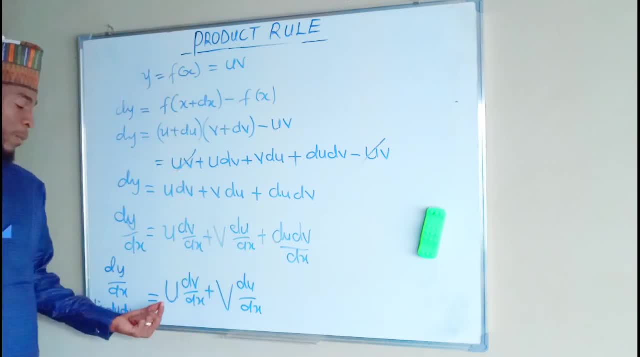 So, in a nutshell, this is what we have: udv over dx plus vdu over dx if the functions are in product form.